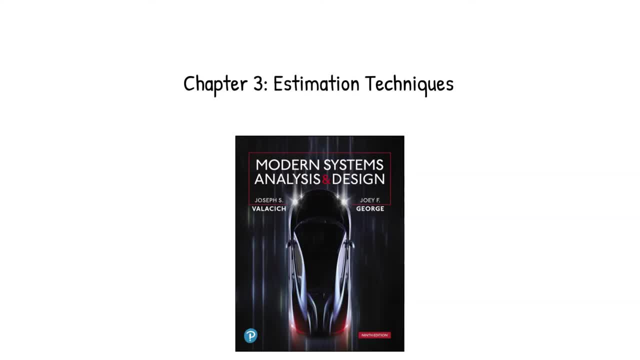 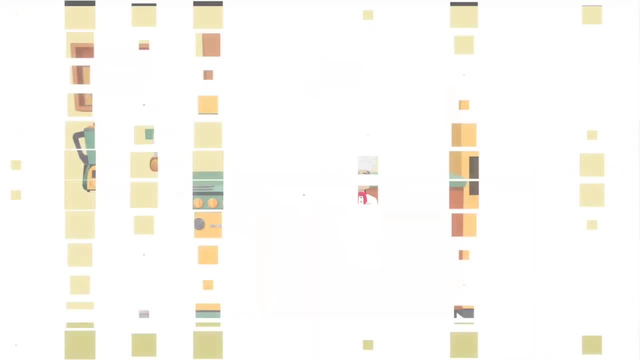 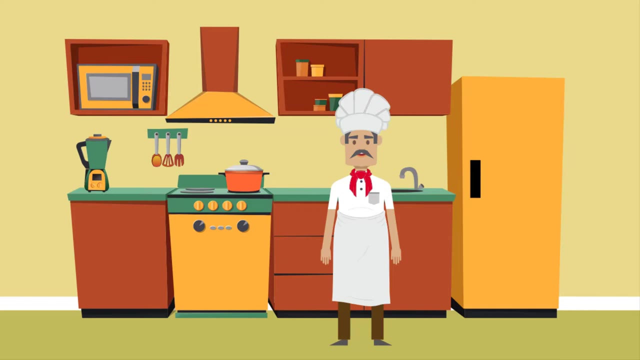 It all depends on your experience in the field, the size of the project, your available resources, mother nature and plain old-fashioned luck. Three ways of estimating time are bottom-up estimations, top-down estimations and three-point estimations. 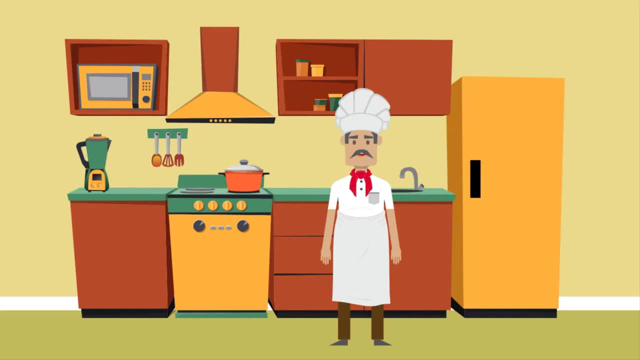 Bottom-up estimations come from knowing what kinds of tasks you plan on including in the overall project and estimating how long each of those tasks will take. From there, you can determine how long the overall project will take. If you're making dinner, you can estimate how long each dish will take to make before saying to the family that dinner will be served in two hours. 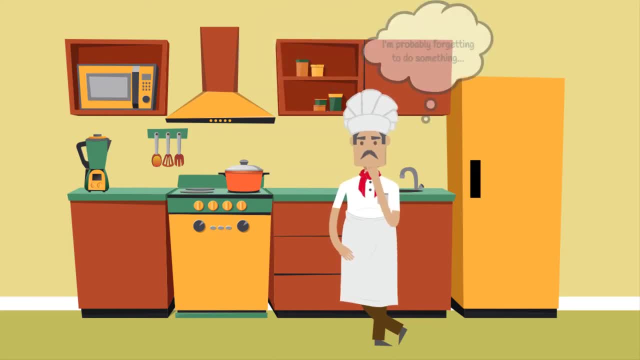 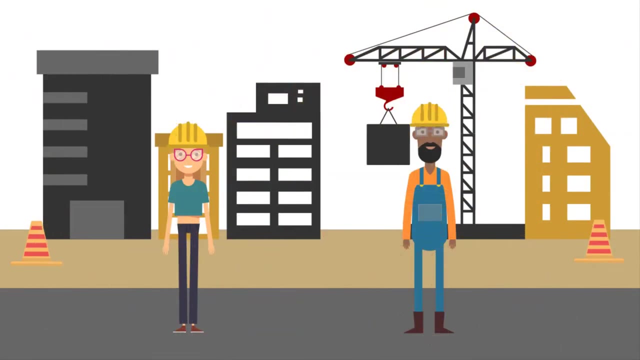 If you're building a house, you can estimate how long it will take to pour a foundation, put up the framework, put the roof on, put up drywall and finish the interior and then come up with an overall time estimate based on the individual time estimates. 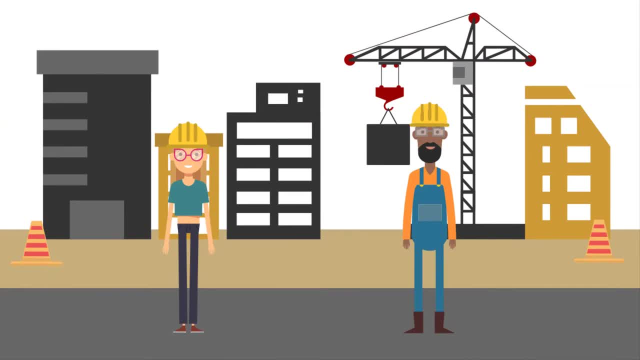 Top-down estimates, on the other hand, are estimates for the entire project. These estimates are usually based on previous or similar projects. If you know how long a similar project takes to complete, you can adjust that estimate based on the time of the project. If you're building a house, you can estimate how long it will take to pour a foundation, put up the framework, put the roof on, put up drywall and finish the interior and then come up with an overall time estimate based on the individual time estimates. 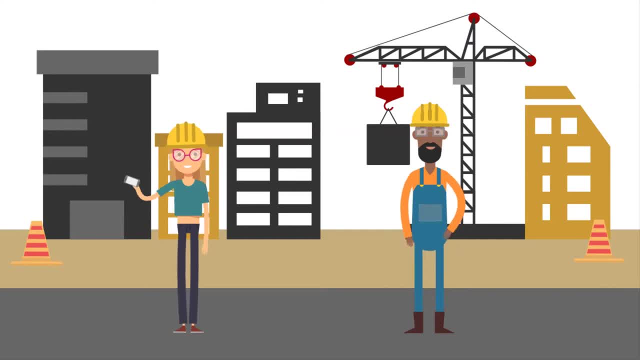 You can adjust that estimate based on the size and scope of the current one. If it takes about 2 hours to make dinner for the family, it may take 3 if you're inviting another family over. If it takes about a month to put up a 2-story house, it may take 3 weeks if you're putting 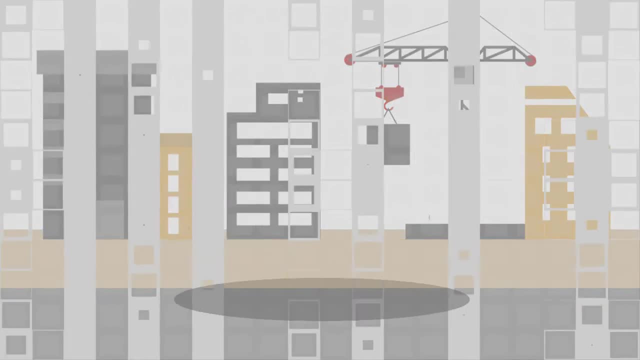 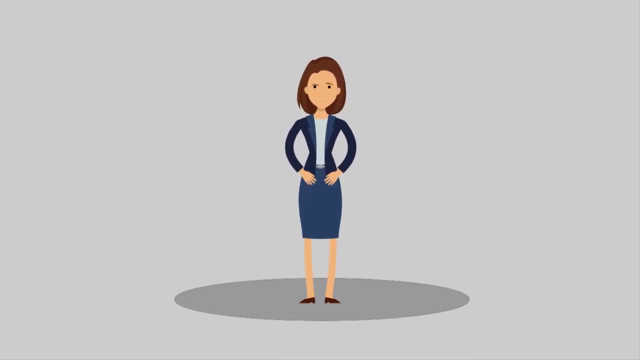 up a 1-story one. Three-point estimations are ways of taking average values to come up with an estimate. With this kind of estimation you want to find the most optimistic estimate, the most pessimistic estimate and the most likely estimate. 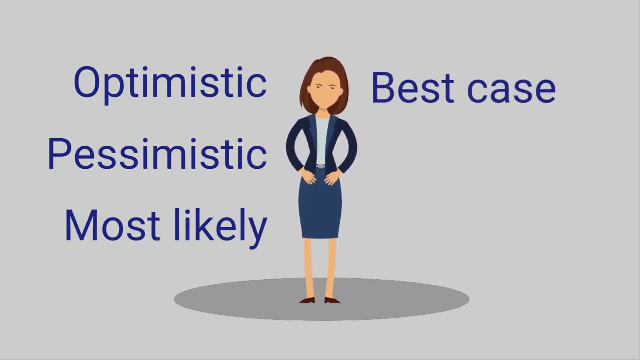 Depending on who you talk to, these may be referred to as the best case, worst case and most probable case. There are two ways of doing a three-point estimate. One way is called the triangular distribution, which is basically taking the average of the.